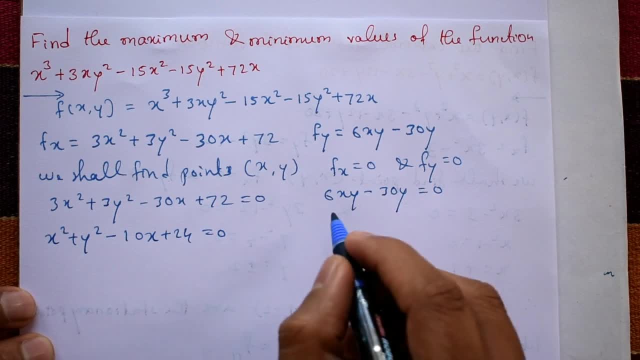 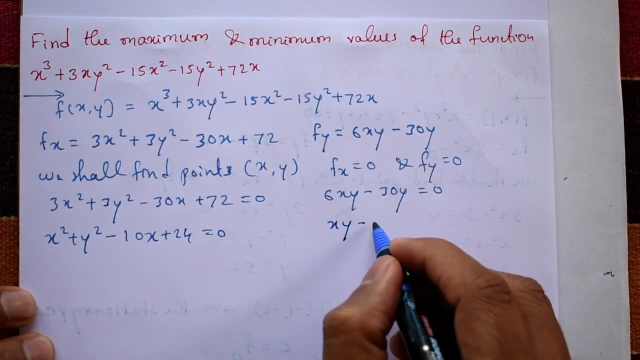 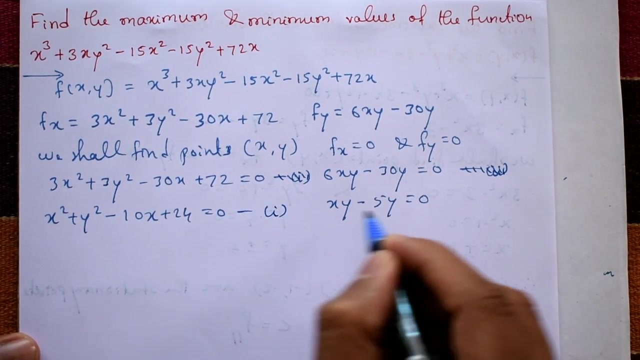 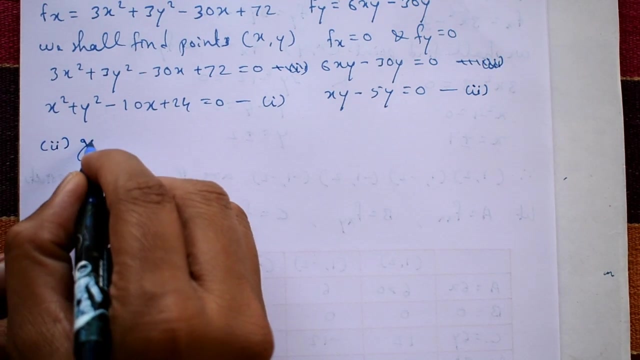 The second equation is divided by 6. Means this is only xy minus 5y, 5y equal to 0. This equation is equation number 1.. And the second one is equation number 2.. Okay, Now equation number 2 gives: 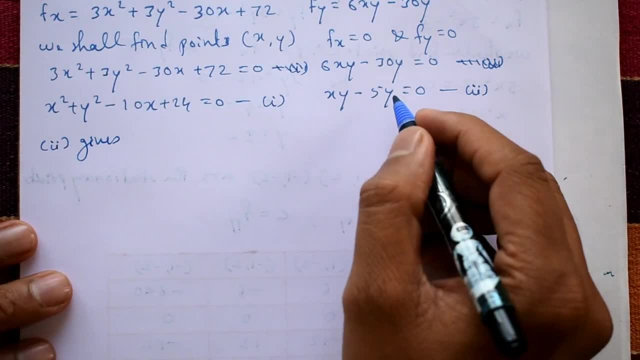 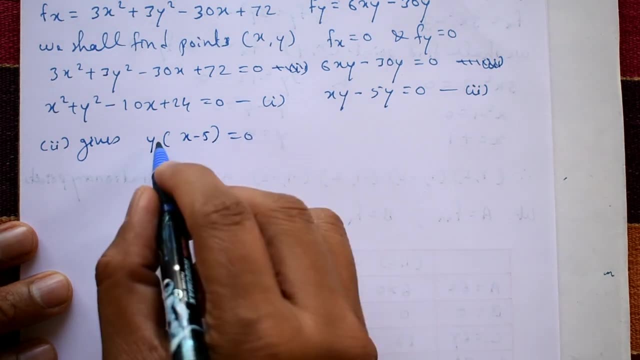 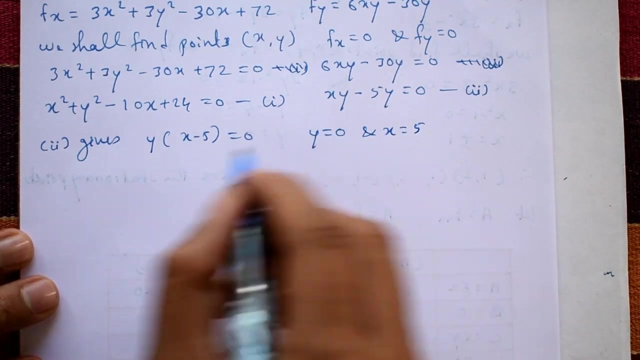 Now see equation number 2.. xy minus 5y- We will take chim bear- y common means x minus y equal to 0. okay, now one is y equal to 0 and x is equal to 5. okay, first take y is equal to 0. putting y equal to 0 in equation number one, this: 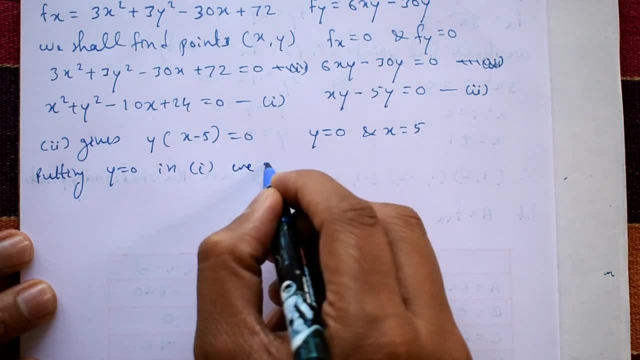 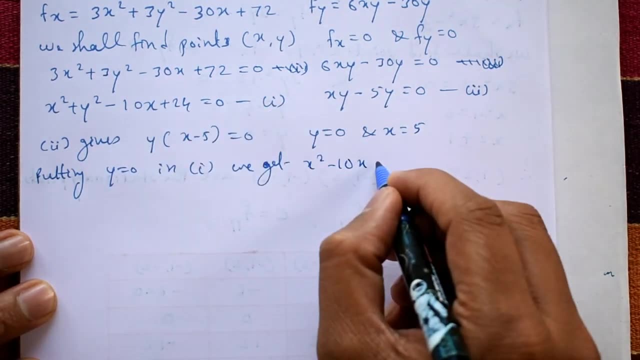 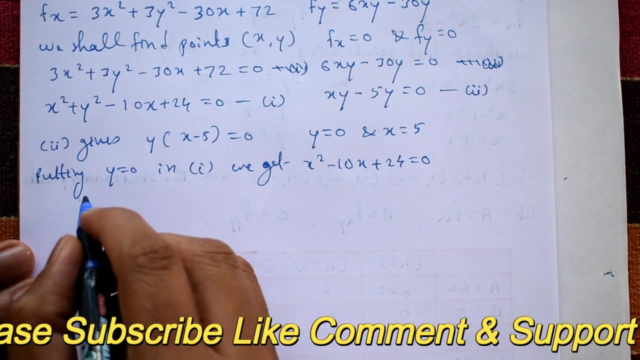 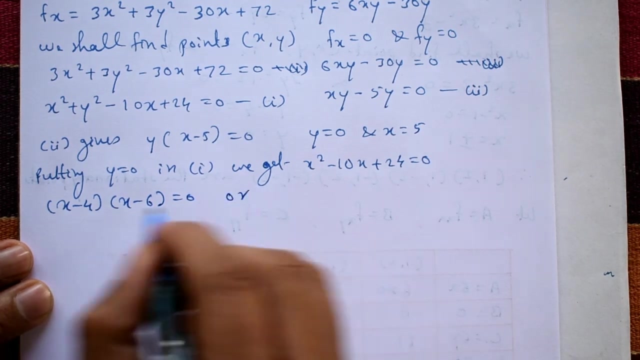 equation number one: put y equal to 0, we get x square y is 0 minus 10, x plus 24 equal to 0. very simple now factorization, factorization this equation: we get x minus 4 into x minus 6. that is equal to 0. so we have x values are: x is 1, is x minus 4 equal to 0 or x is equal to 4? 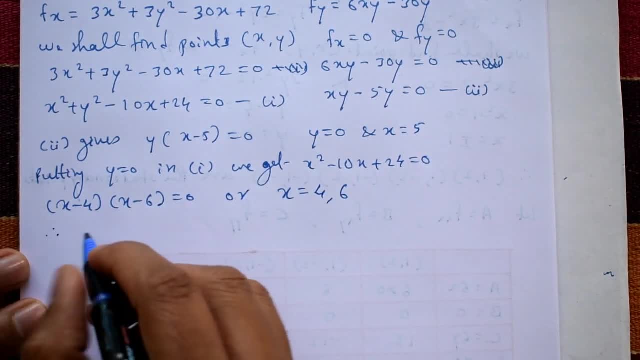 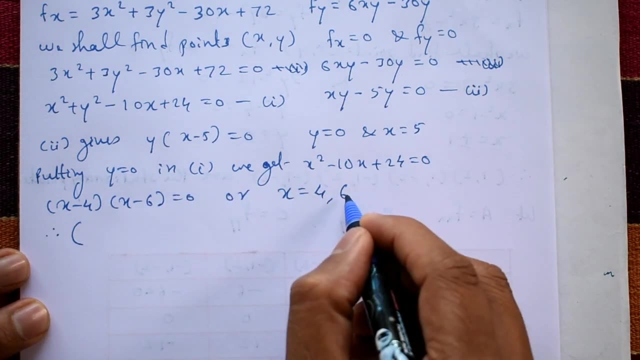 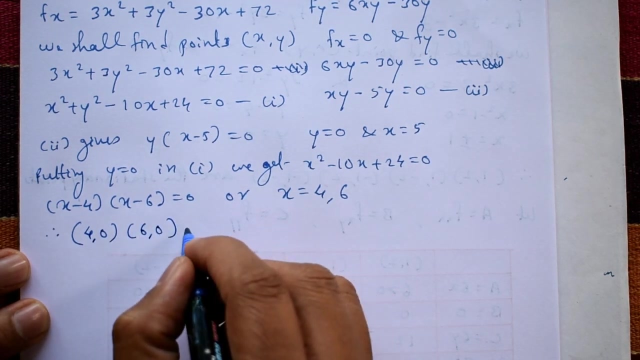 second is: x is equal to 6 now. therefore, now stationary points are: first you take x value and then after y, x is 4, y is 0. second point: x is 6, y is 0 means 4: 0 and 6: 0 are stationary points. 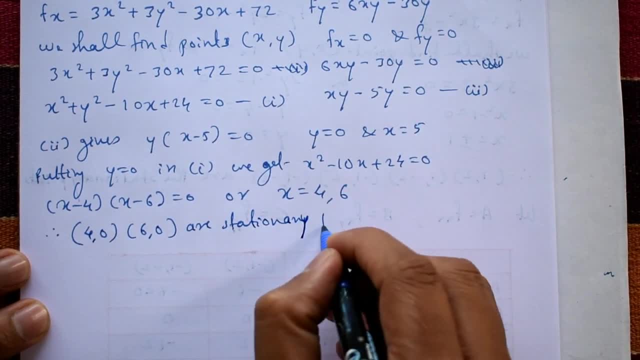 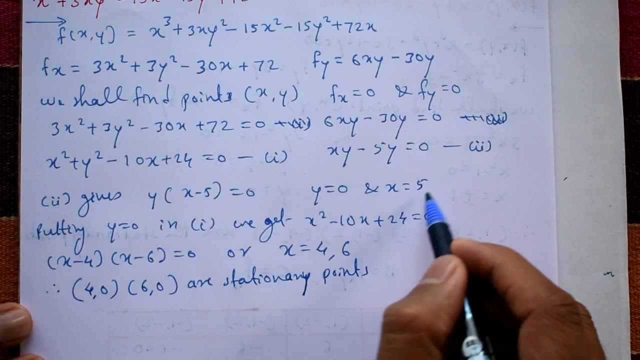 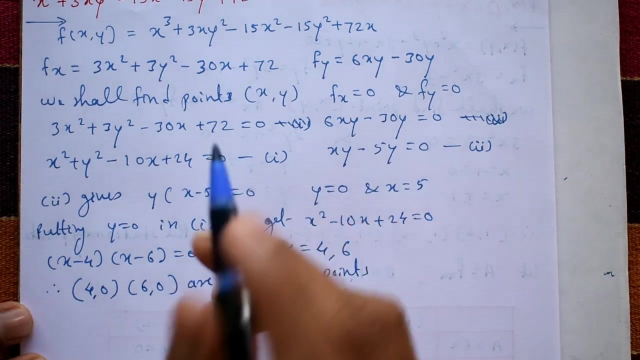 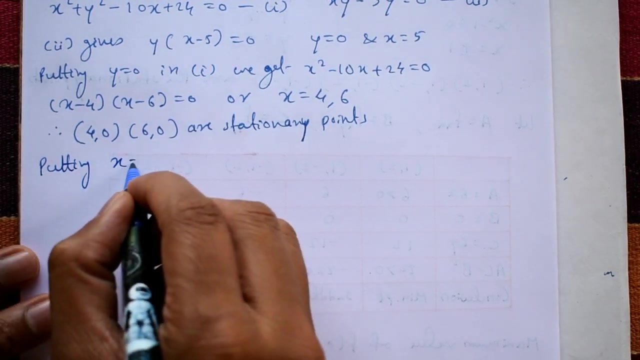 okay, these are. these two points are a stationary points. next, 1, y equal to 0. then take second in equation 2, that is equation 2 gives again x is equal to 5. put in equation number 5 equation 1: take x is equal to 5. now putting x is equal to 5 in equation number 1. 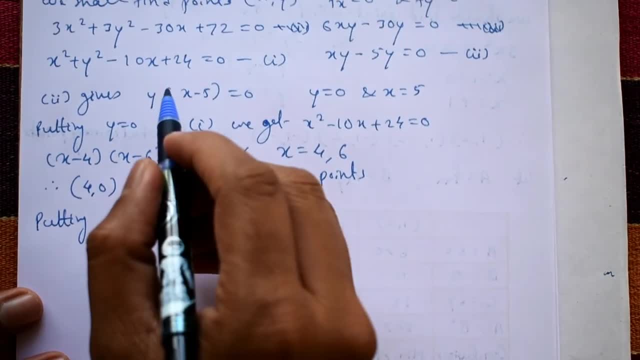 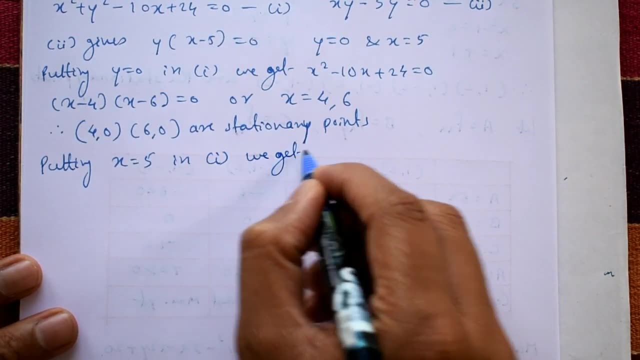 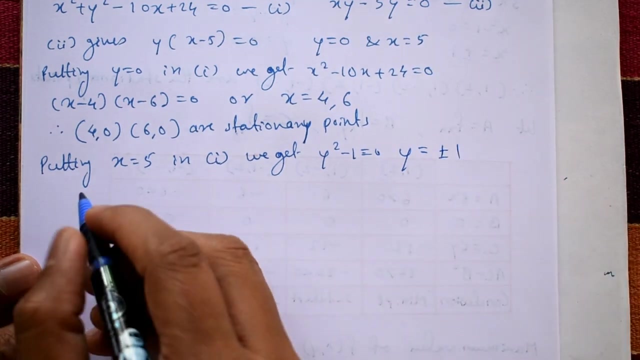 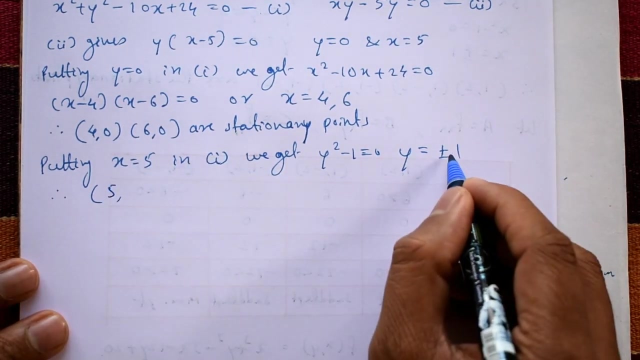 take x is equal to 5, means this one 5, 5. in this equation we get very simple. we get y square minus 1 equal to 0, or y is equal to plus or minus 1. okay, again the stationary points are: take x is equal to 5, 5 minus 1. for you plus 1. we have two points for you, first one. 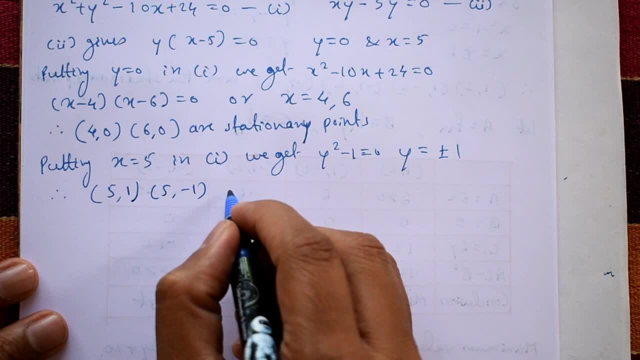 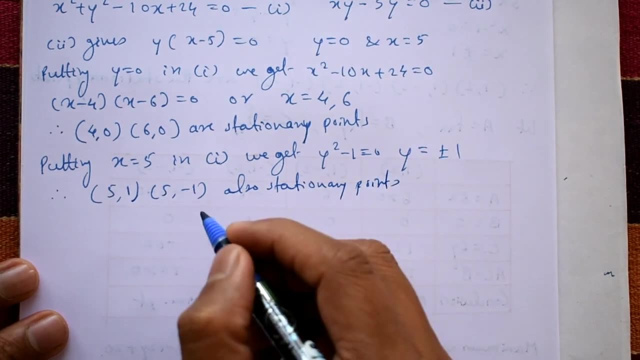 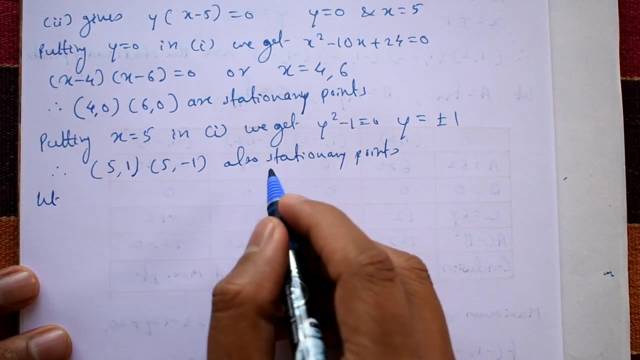 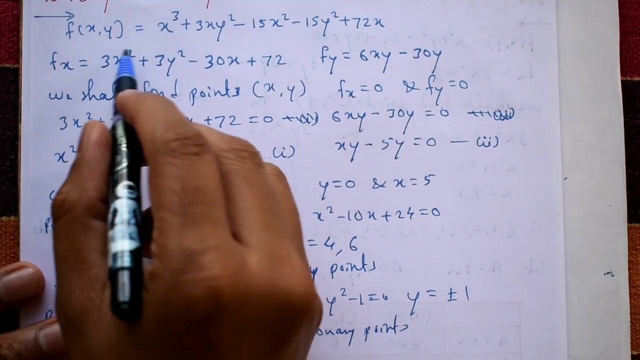 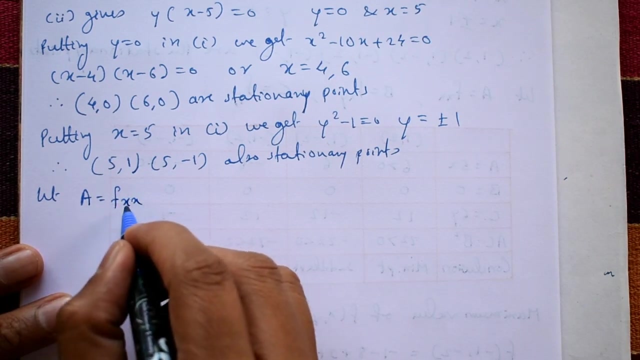 post a positive and for you minus 1. these are a, also stationary points. okay, now, these are a stationary points. now let we find extreme values, these two maximum and minima. now take a is equal to now a means again, differentiate this equation that is a, that is a, with respect to differentiate function with. 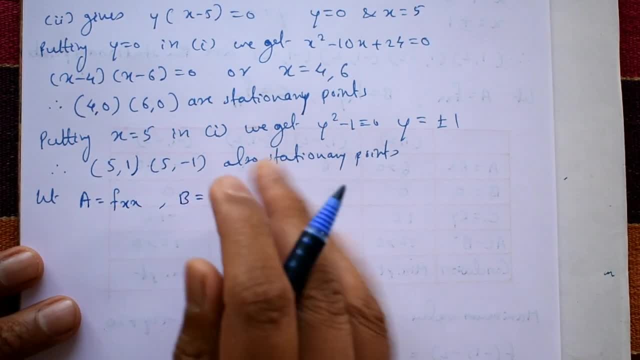 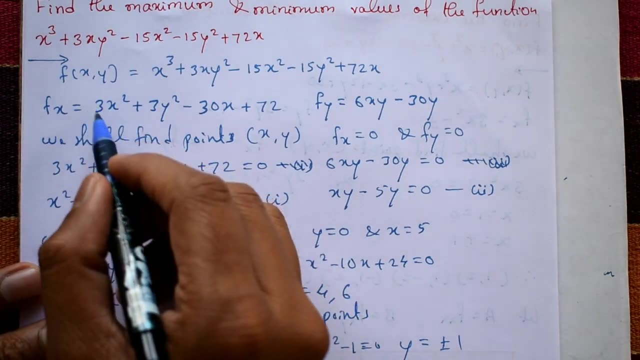 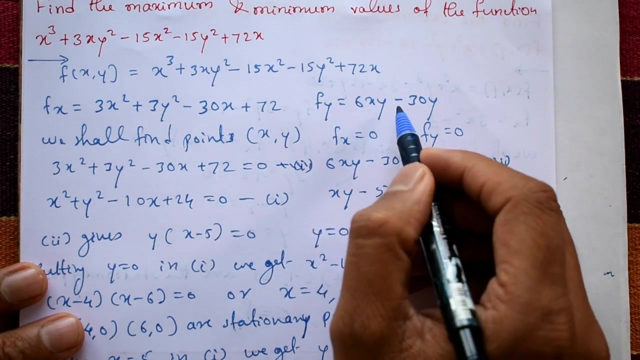 respect x 2 times and take a. b is equal to b means take any one. okay, first time with respect to x is over, then second time with respect to y. or consider second equation: first time with respect to y is over, then take, second time with respect to x. take any one we. 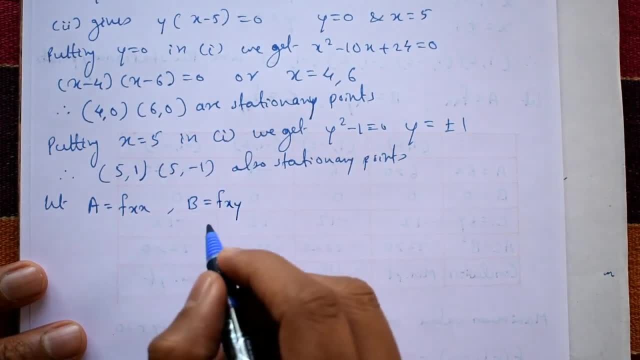 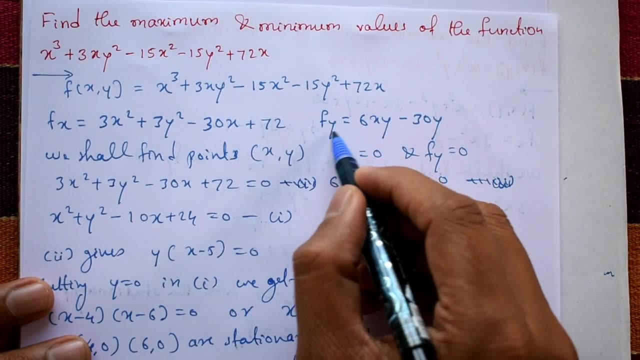 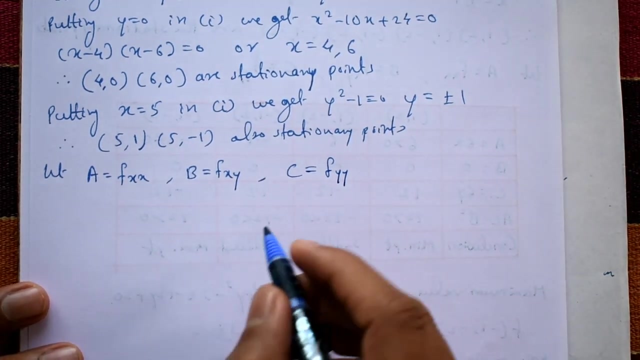 get same result means x and y or y and x. we get same result. now c. c means consider this one with respect to y. y is over, once again with respect to y. partially you get do f, y, oh, with respect to y two times now. table is now. take stationary points now: a, b, c, a, c minus b square. 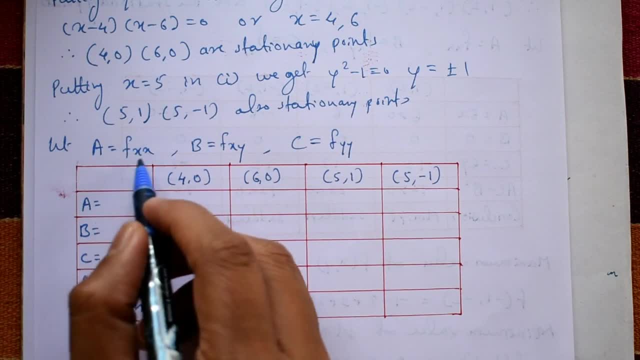 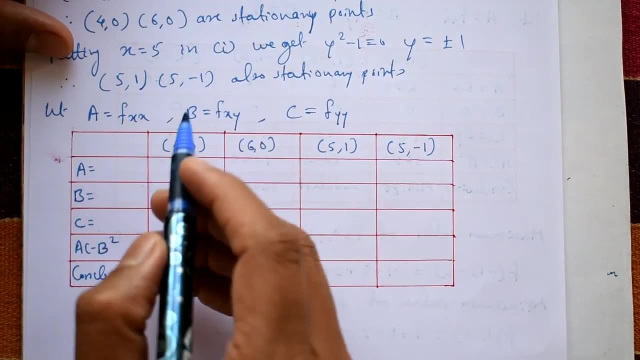 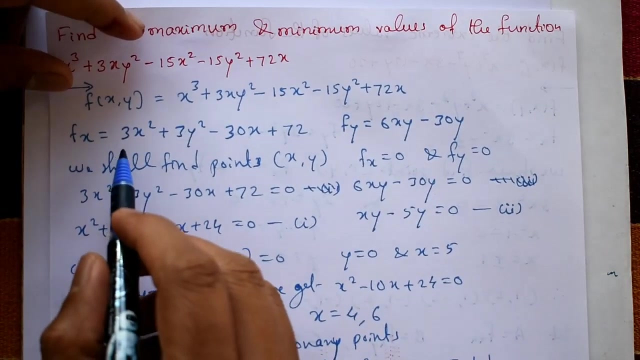 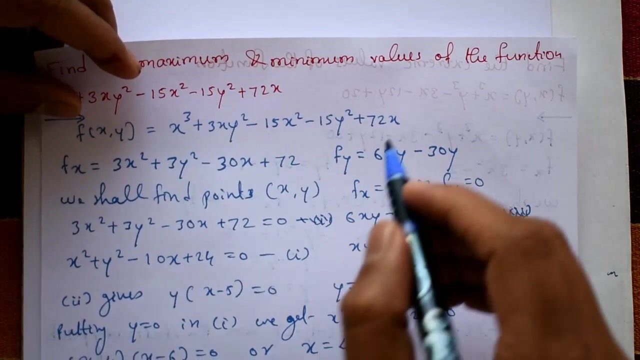 and conclusion: a means differentiate function with respect to x. two times means again differentiate. this one we get, a is equal to that is a 6x minus 30. now b means take any one with respect to y, or consider this one with respect to x. we get b is a 6y only now take. c means second one with 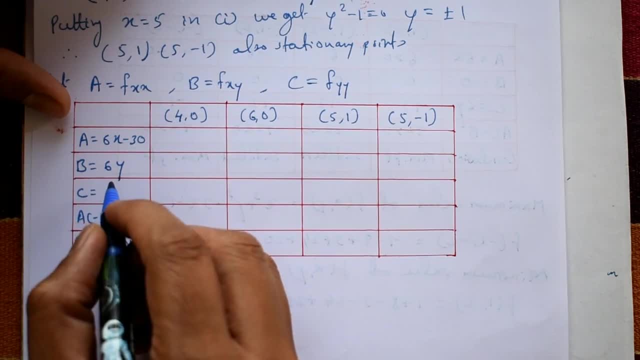 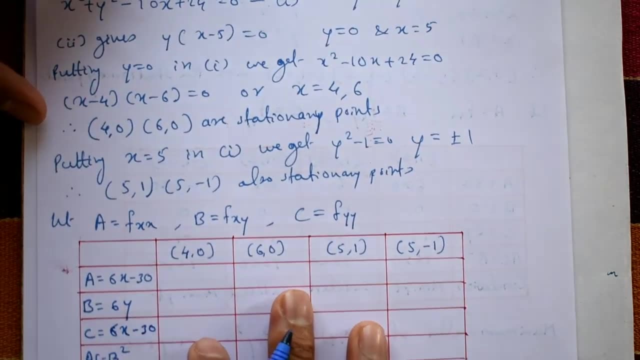 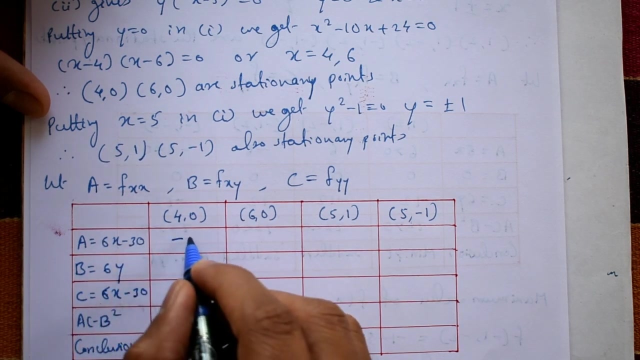 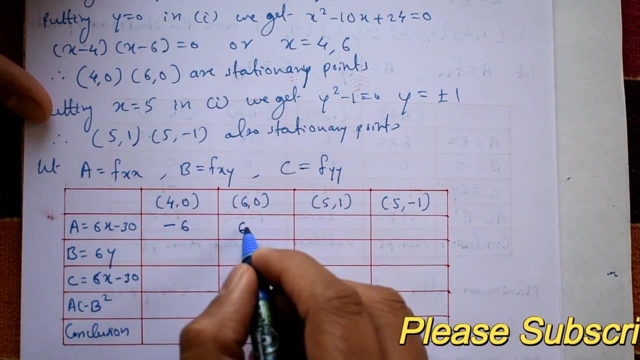 respect to y once again means two times. with respect to y, c is equal to 6x, so minus 30. okay, now take x and y values. put x values in this one: 24 minus 30 is a minus 6. put x values plus 36 plus 36 minus 30 plus 6. put x and y values, we get 0. put x and y values: 0. 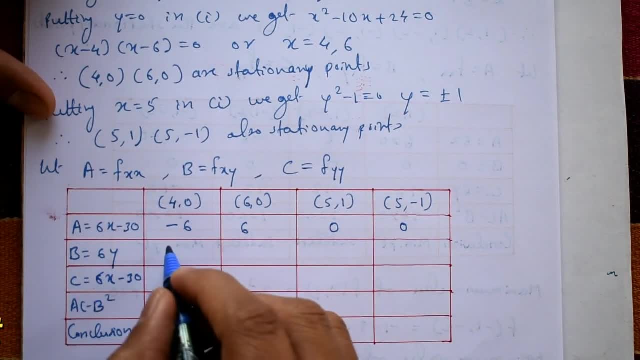 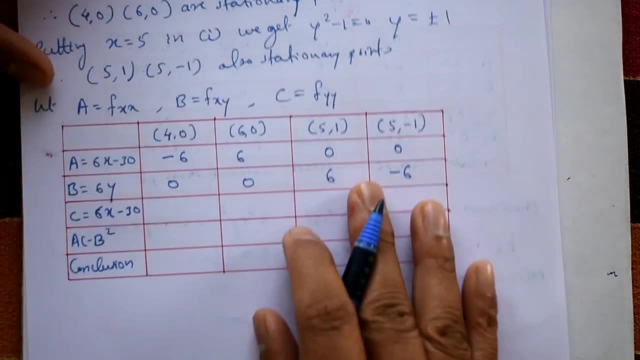 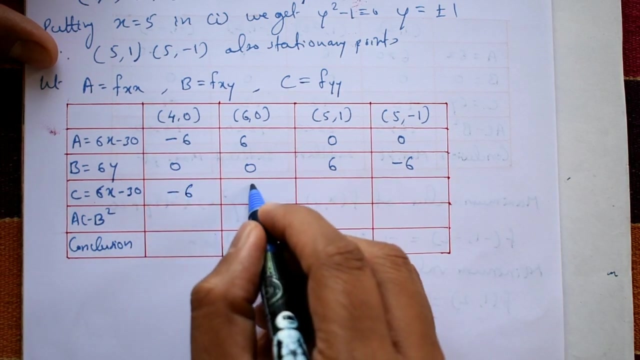 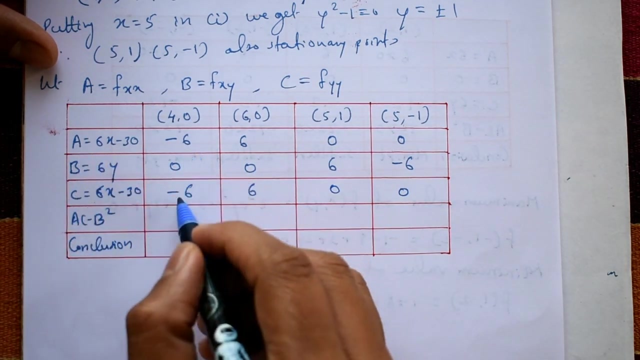 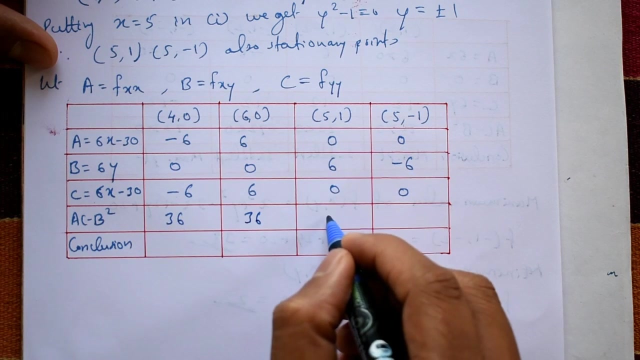 now second one: b is equal to 6y put values 0, 0, then 6, then minus 6. okay, now put these values, x and y values, in c, you get minus 6, 0, 6, 0, 0, a c minus b. square a into c plus 36. b is a: 0 plus 36. multiplication plus 36: 0 minus b square. 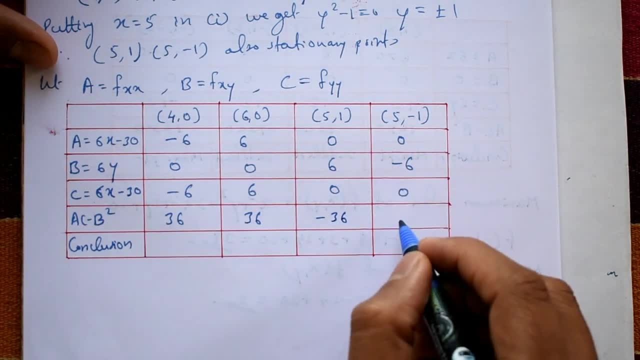 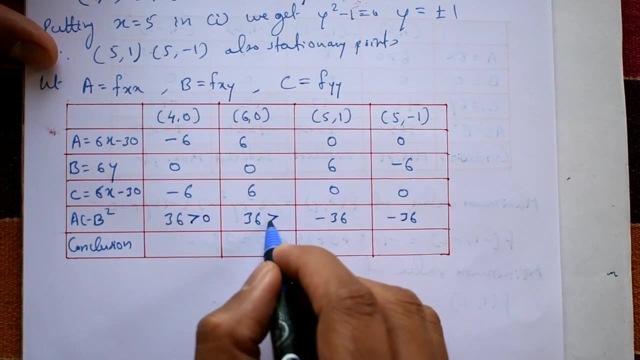 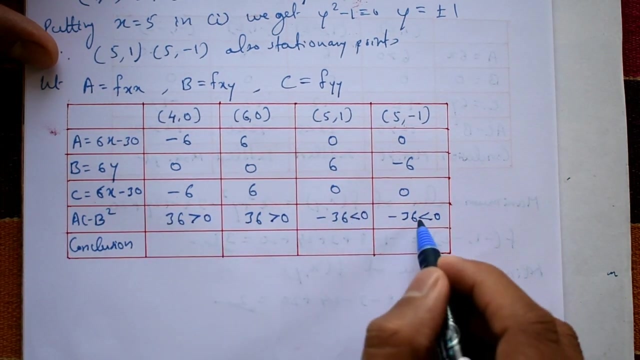 means minus 36. same, it is minus 36. now see the a, c minus b square. this is positive. this is positive. now, this is negative value, negative value. now see these two point: these put these: a, c minus b square less than 0 or equal to 0. that point is saddle point. 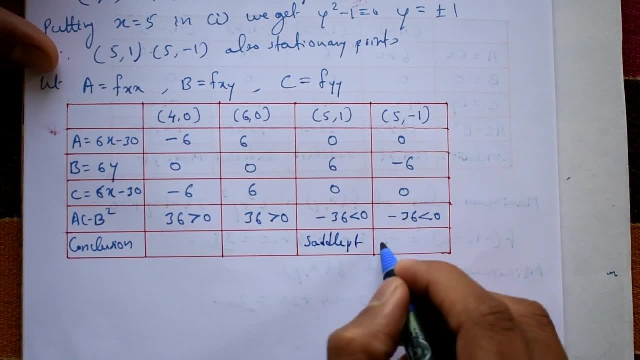 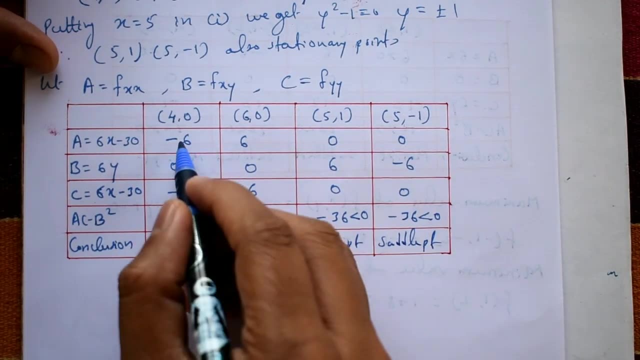 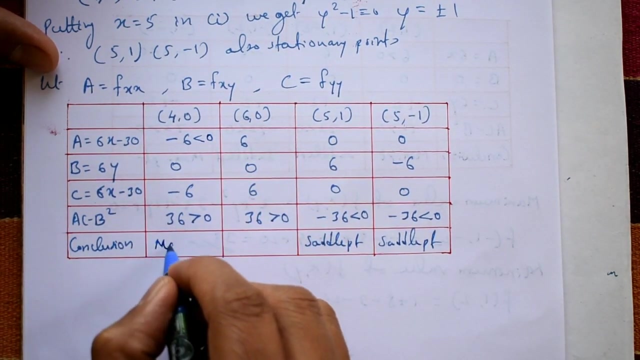 directly mention saddle points. this is also saddle point. now see this one: a, c minus b square is greater than 0. now check a value. these values are greater than 0, but a is less than 0. that is a maximum point. okay, now a, c minus b square is greater. 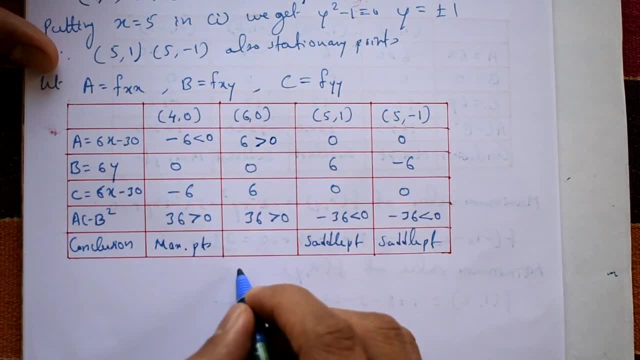 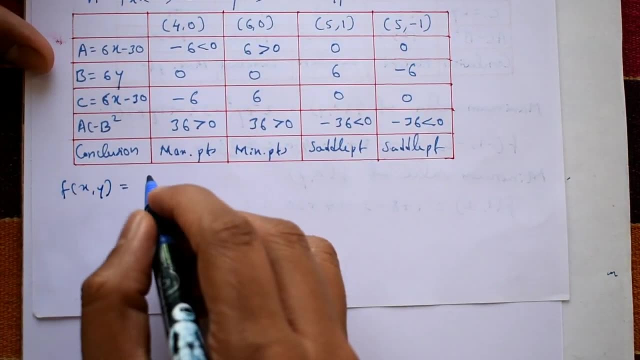 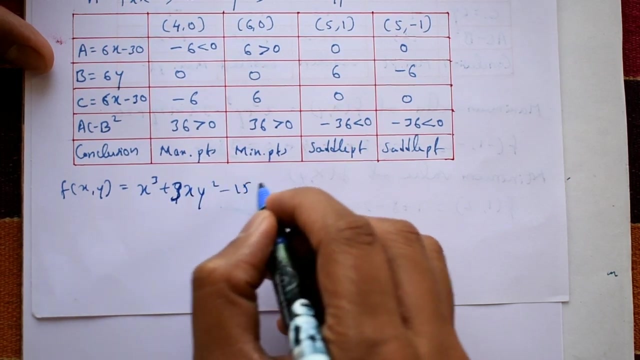 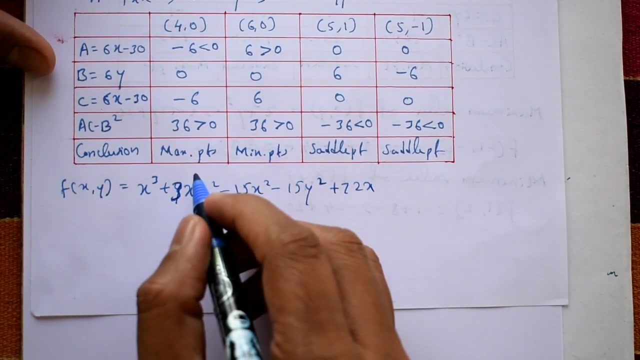 than 0, but a value is positive, greater than 0. now this is minimum value, minimum points. okay, now we have a f of x. y is given x cube plus 3, x, y square minus 15. x square minus 15. y square plus 72, x. now find maximum value and.